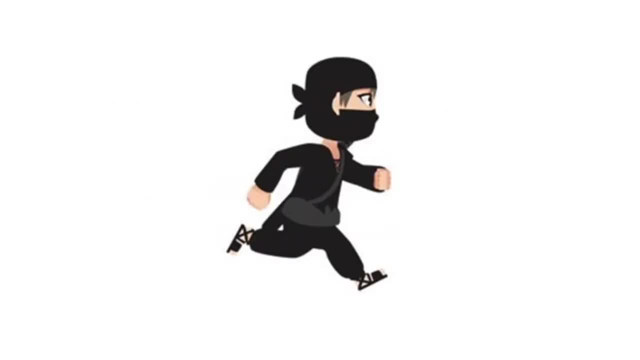 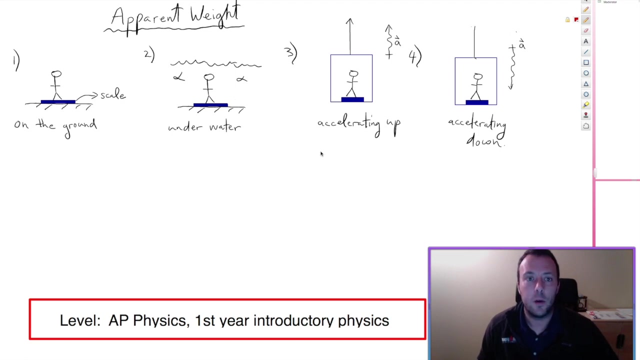 Today I'd like to talk about apparent weight and problems that deal with apparent weight. I came up with six examples: four on the first page, two on the next page. that are different situations where you might be asked to calculate the apparent weight. So the first thing we 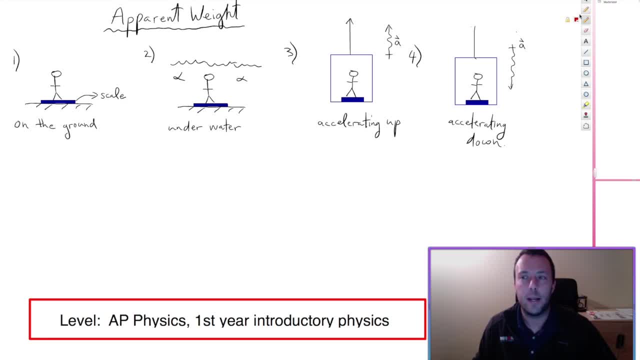 have to do is you really have to define what apparent weight means to you. It's not complicated. Whenever someone asks you to find the apparent weight in any kind of problem, just remember that the apparent weight is basically the normal force, That's, the force of the scale. 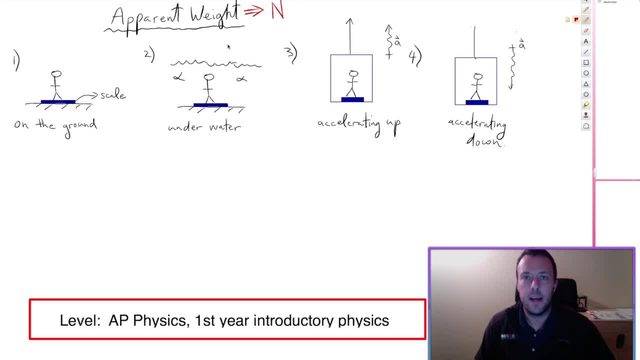 Imagine you're standing on a scale in each one of these situations and it's the force that the scale is producing on the body. So let's take the easiest situation here, just the person standing on the ground. If you do a free body diagram on that person again, 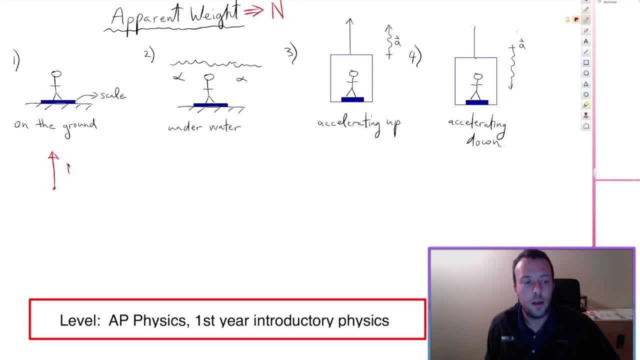 there's a normal force here and what else. There's also going to be a weight. In this case it's a mass of the guy. times little g Again, if this guy is not accelerating. that's a very simple problem to solve. You get the. 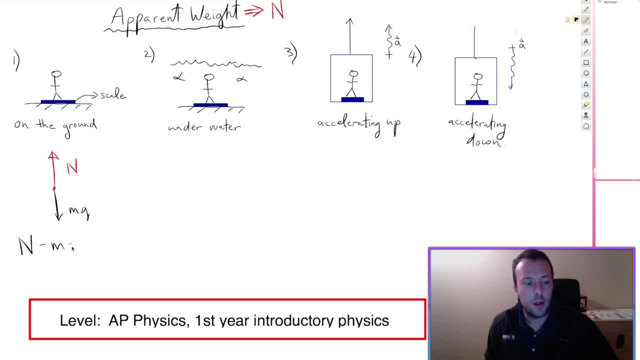 normal minus the weight has to be equal to zero. I've added all the forces and there's no acceleration in this case. so we get the simple answer that the normal or the apparent weight- in this case it's not really apparent, it does- equal to the weight. That's case number. 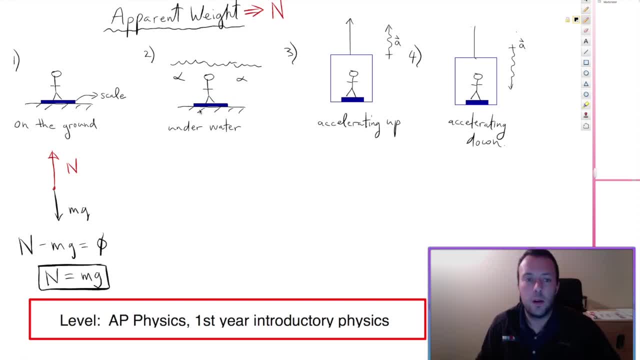 one. Okay, what about case number two? Well, what if you're standing at the bottom of a pool, and again you're standing on a scale and you were asked to calculate the apparent weight? Well, again, when you're at the bottom of the pool, you still have the weight which has a magnitude of mass times, little g. What? 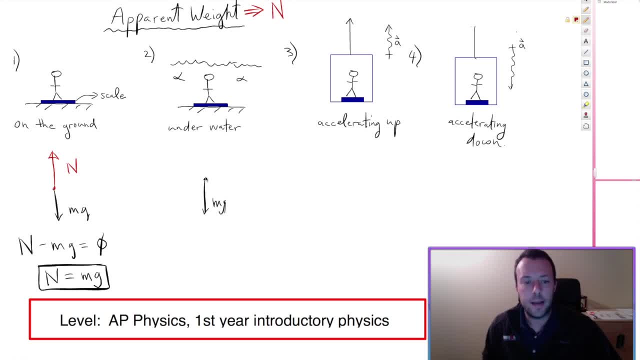 else We're going to have a normal force. that's the scale pushing up on the guy. call that n. And there's also another force now. So when I'm displacing fluid, there's also a buoyancy force, and I'll just call that b. 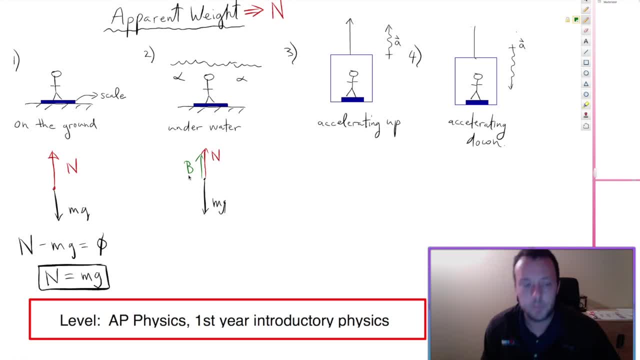 And the buoyancy force is in the same direction as the normal force. Okay again, if there's no acceleration for this object, if I'm just standing here at the bottom of the pool, all of these forces have to sum to zero. Okay, so we simply have. 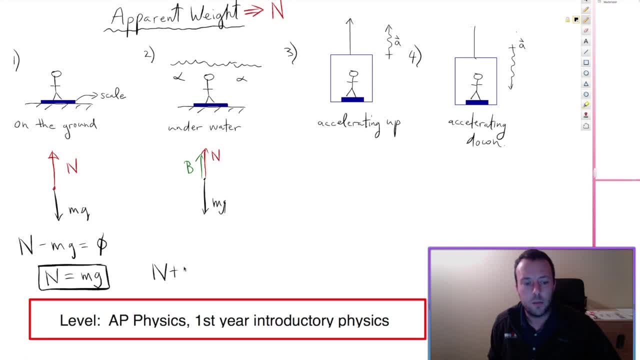 that the normal minus… Sorry, Plus the bool buoyancy force has to be equal to mass times little g. Now if you simplify this a little bit, just bring the buoyancy force on the other side, what do we get? That the normal force is equal to mg minus the buoyancy force. So here's. 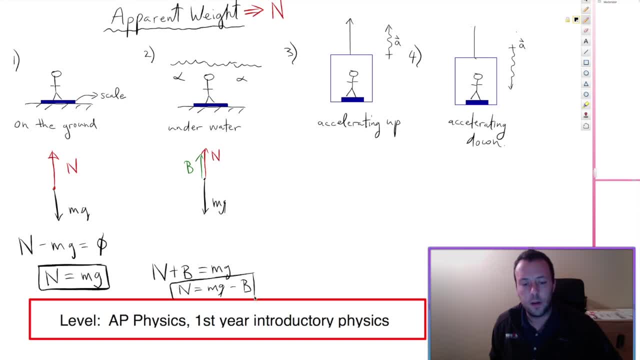 our expression for the apparent weight when an object is at the bottom of the pool. Notice that the normal force, in this case the apparent weight, is smaller than case number one. Okay, let's take the next case now. Again, we do a free body. 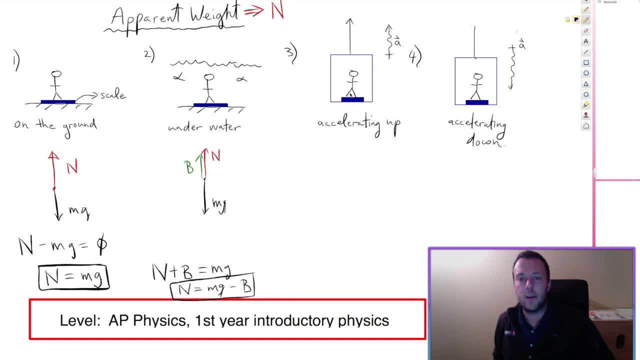 diagram. This is someone standing in an elevator on a scale, and the elevator is accelerating upward. Okay, we're going to do our free body diagram here. That guy still has the same weight Whether he's standing on the ground, whether he's underwater or whether he's. 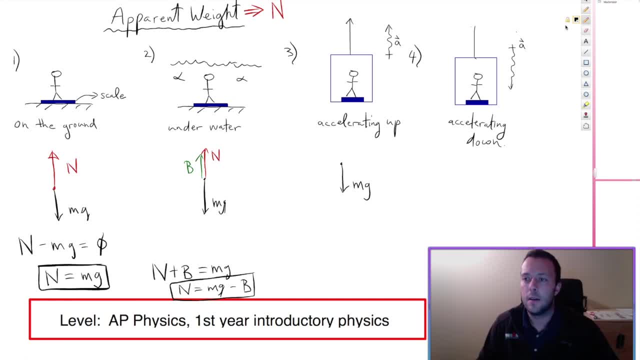 accelerating up. that doesn't change how much mass he has. The next thing we have is there's a normal force. He's standing on a scale, So that's going to have a reading And that's it. Those are the only two forces acting on him. Now, you may be. 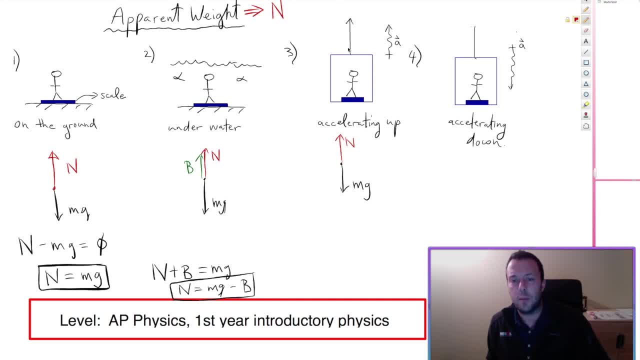 tempted to put this force here, this tension force in the cable. However, that tension force is not acting on the object, It's not acting on the person here That's actually acting on the elevator case And right now for the free body. 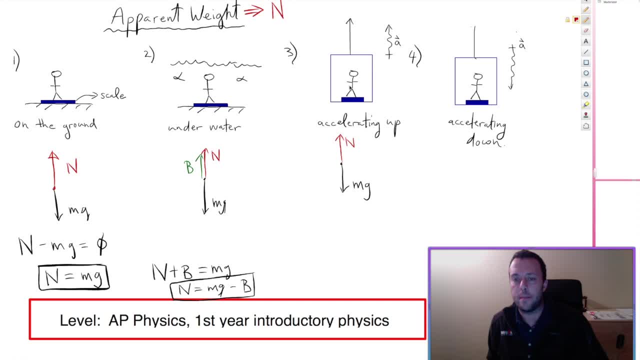 diagram, we're only considering this guy and all the forces acting on him. I've also told you, in this case, that he's accelerating up. Okay, so Newton's second law says you add up all the forces and those are equal to mass times. acceleration: Whenever you have an acceleration, I find it's always best to 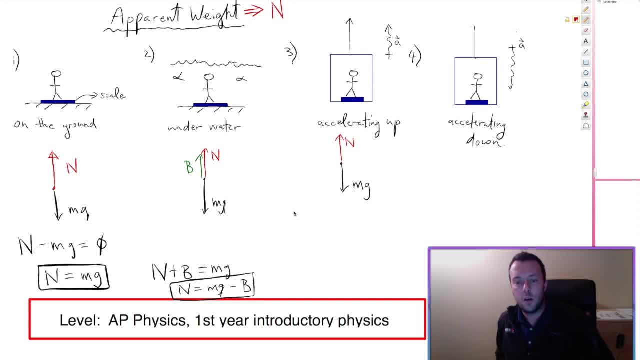 choose the direction of the acceleration as the positive direction. So if we do that, what are we going to get? Switch the colors here You get that the normal force which is acting up minus mg which is acting down has to be equal to mass times acceleration. 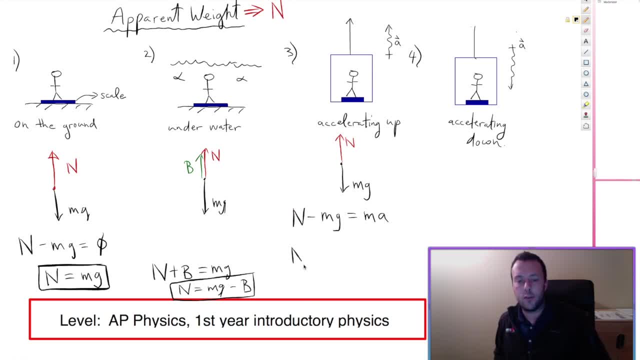 Okay, again, just as I did before, I'll isolate. I get that the normal force is equal to mass times, acceleration plus mass times, little g. You could see in this case again, If I just isolate or take out the mass, I get a plus little g in the parentheses here. 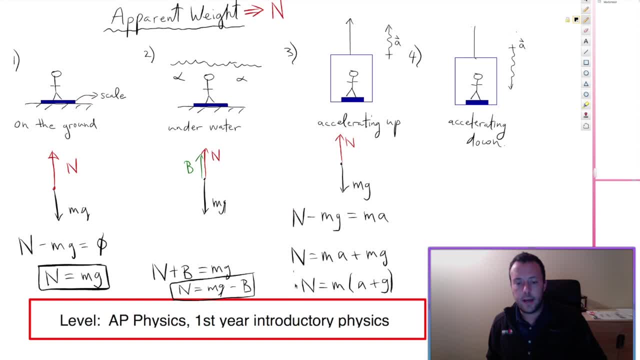 So when I'm accelerating upward, notice that the normal force or the apparent weight of the object is going to be greater than case a. when I'm just standing still, And the faster I accelerate, the bigger this term is, the larger the apparent weight of the object. 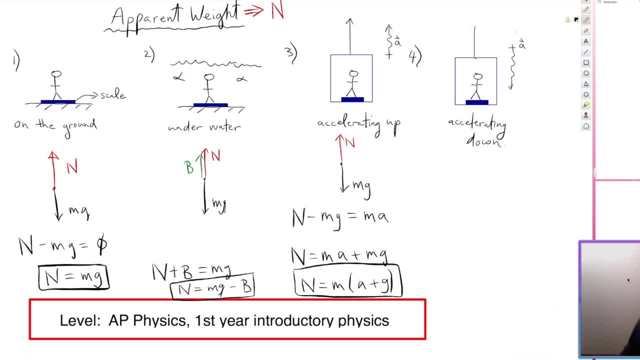 Okay, All right, let's try the last case now. The last case is the same situation as number three, except this case I'm accelerating downward. So the free body diagram actually looks the same thing. The only difference is I'm accelerating downward. 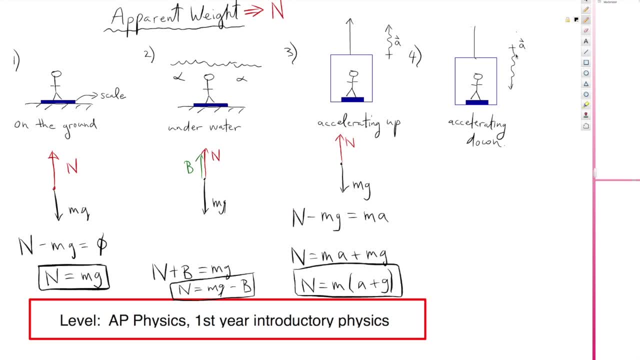 So in this case it's best to choose a. I'll choose the positive direction as being toward the direction of the acceleration. So when I write down the Newton's second law of motion, what I get is mg minus the normal equals to positive ma. 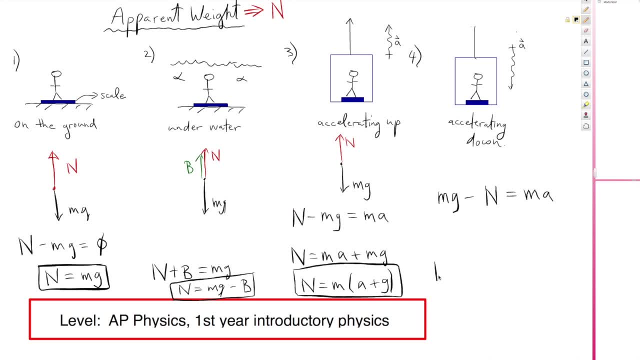 Okay, Now again, if I isolate for the normal force, what do I get? in this case, I get that the normal force equals the mass and little g minus the acceleration- acceleration. So notice, if I don't have any acceleration, I get the same result. 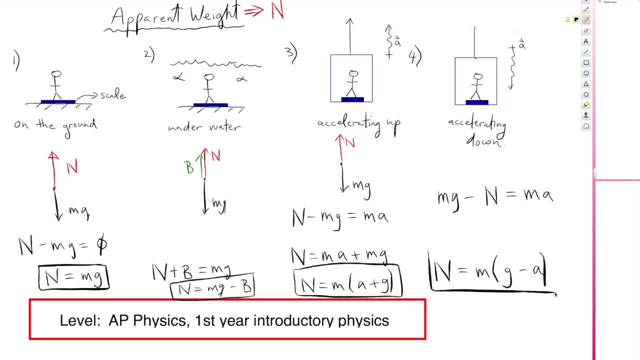 as in case one. So if I'm moving at constant velocity, for example, I get that the apparent weight is simply equal to the weight, but if I'm accelerating downward, notice that my apparent weight is going to be smaller than the weight if I'm just standing on the ground. Okay, so I've got two more cases on the. 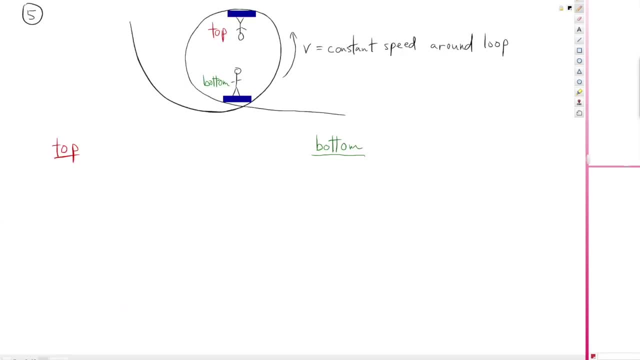 next page. Okay, and here they are. Imagine: here I'm standing on some kind of board and I'm going around a loop-de-loop like this and I want to find what is the apparent weight at the top and what is the apparent weight when. 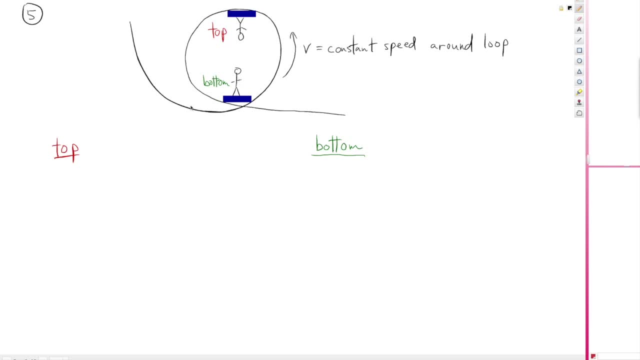 I'm at the bottom. Okay, for this problem here, we're going to just assume that the velocity is constant throughout the entire trajectory. the speed is constant rather than the velocity. So if I'm going to go to the next page, I'm going to 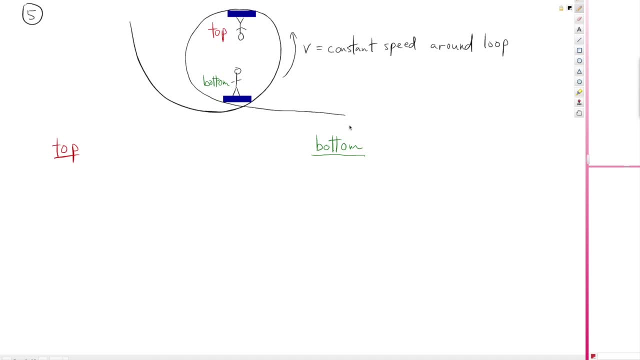 find what is the apparent weight of the top and what is the apparent weight of, but the velocities constantly change in direction here as I'm going around this loop. Okay, so let's see what's going on at the top. At the top, if you look at all the forces acting on the object, it still has a weight which is mg. 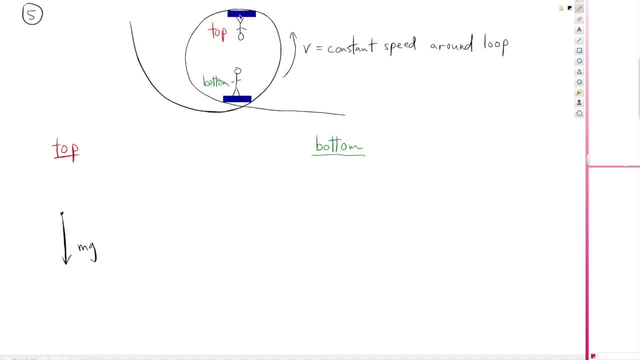 And now the normal force or the contact force, the force from the block acting on the guy, ends up being in the same direction as the weight. That value is n. Now you should know that when you're at the top, the direction of the acceleration- again, if I'm going around in a circle here- when I'm at the top, the direction of the acceleration. 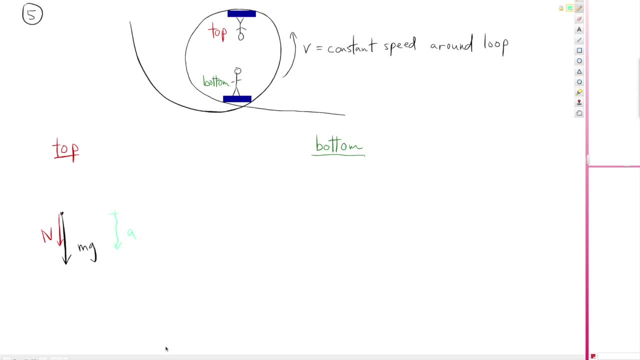 is toward the center of the circle, That's the centripetal acceleration of the object. Okay, So let's look at the bottom case now, The free body diagram for the bottom case. Well, that just looks like a regular free body diagram that we're used to doing. 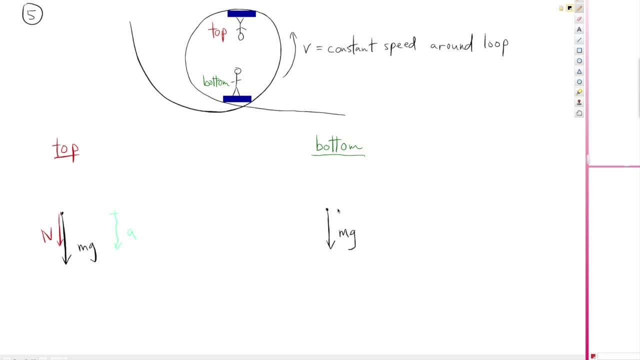 Yep weight acting down, which is the same for every single case we've seen, and you have a contact force. Now this block is pushing up on this guy. That's the normal force, or this contact force between the block and the person, And that's it. Those are the only. 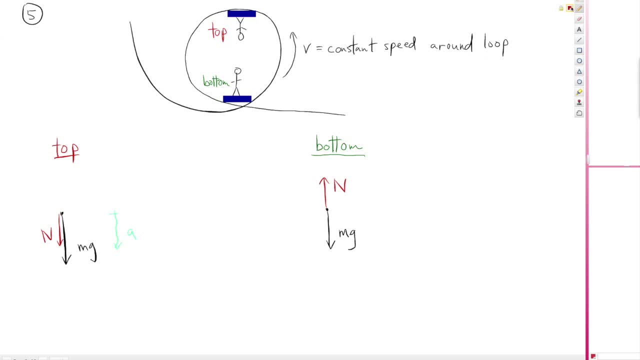 two forces acting on the object. Now, the only difference from the top and the bottom is that when I'm at the bottom, I know that the acceleration is toward the center of the circle, And when I'm at the top, the acceleration is toward the center of the circle, but acting 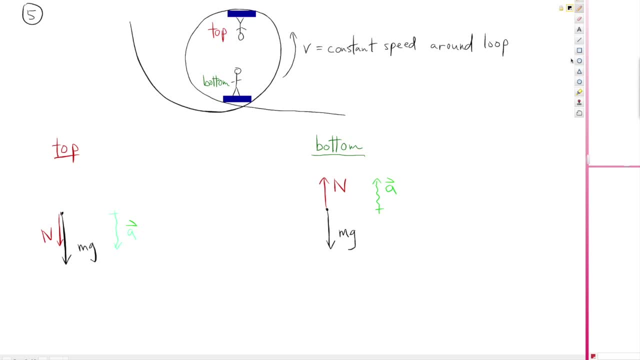 down. So all we need to do now is just apply Newton's second law to both of these problems. At the top we're going to have the normal plus mg Equals to mass times acceleration. Since I'm going around at constant speed, that acceleration. 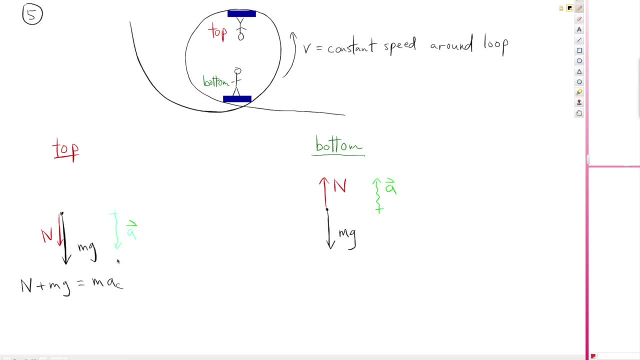 takes this very specific value, this centripetal acceleration. So I can rewrite that centripetal acceleration as mv squared divided by the radius of the circle. Okay, if I isolate for the normal force, which is what I'm trying to find here, that's the apparent weight I'm going to get. 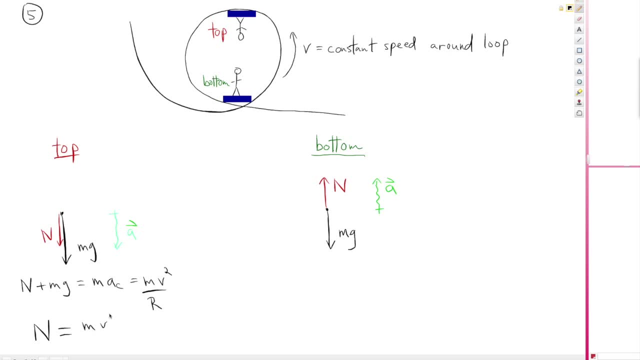 mv squared over r Minus mg. And here's my expression for the apparent weight when I'm at the top. Let's compare that now to the case when I'm at the bottom. Okay, when I'm at the bottom, I'm going to apply Newton's second law Again: the acceleration. 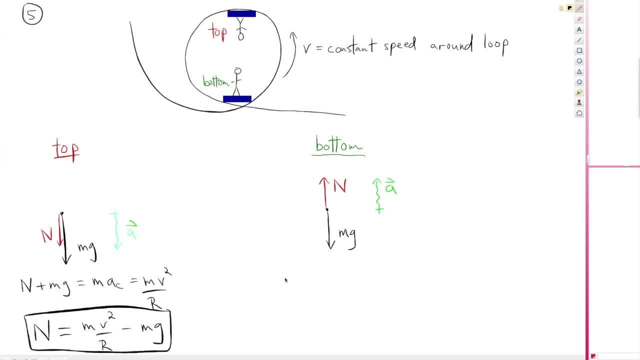 is toward the center of the circle, so I'm going to take that to be my positive direction. So if you apply Newton's second law, you'll get normal force minus, mg minus because it's acting away from the center of the circle, And again that equals to mass times, the centripetal 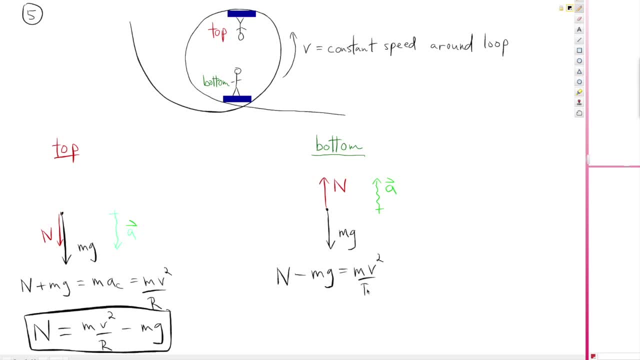 acceleration, which is v squared over r. Okay, so the normal force here when I'm at the bottom, if you isolate, you get mv squared over r plus mg. Okay. so first thing we notice is that, in the case for the bottom, notice these two: 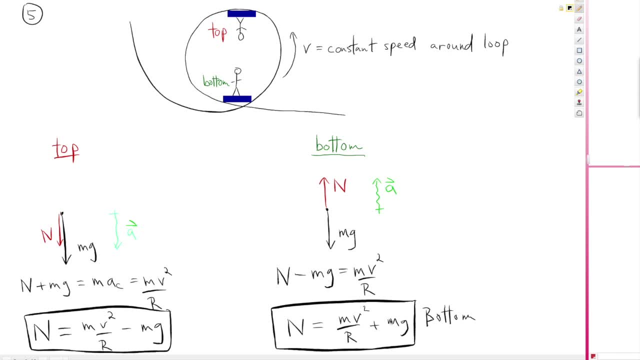 terms are always adding together, So I'm always going to get a bigger apparent weight. when I'm going around in a circle at constant speed and I'm near the bottom, In that case the normal force has to be bigger than the weight. The normal force must be.